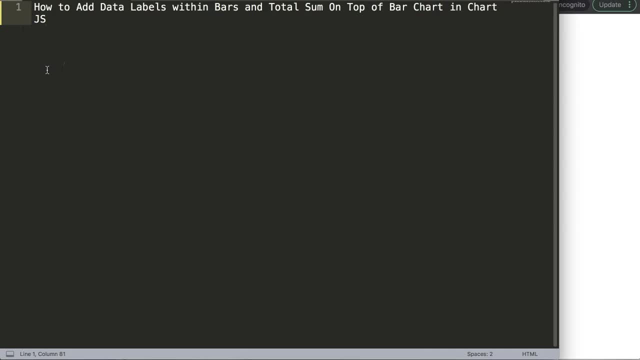 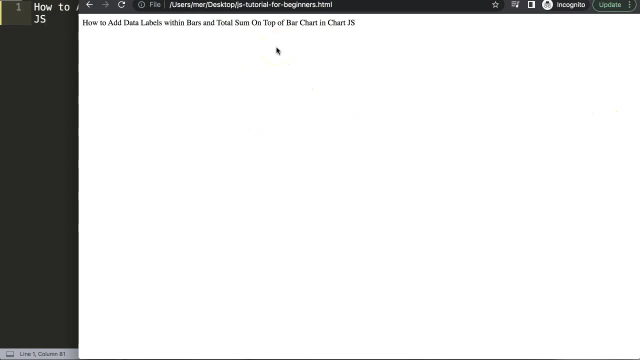 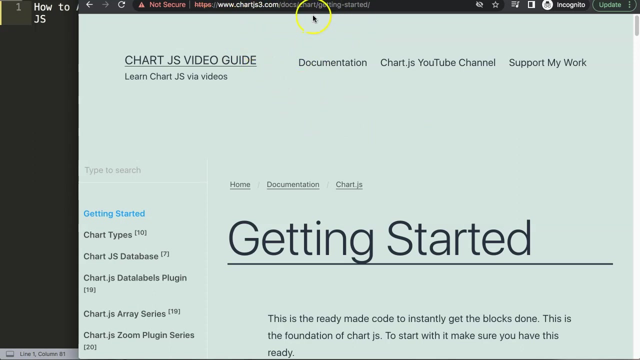 So let's start to look how to add data labels within the bars and a total sum data label on top of the bar in a bar chart in Chartjs. So the first thing, what we need is, of course, to have a default code. so for that we can find it on Chartjs3.com getting started, or this specific link here, which you can also find in the description box. 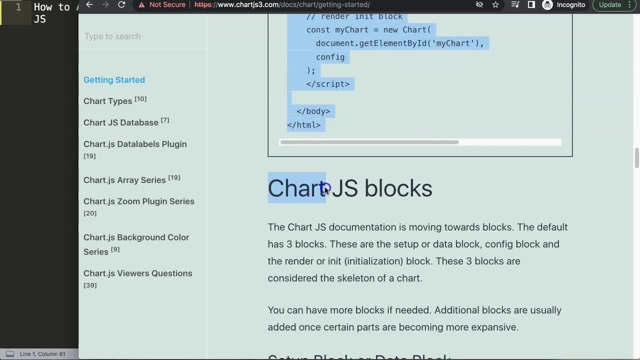 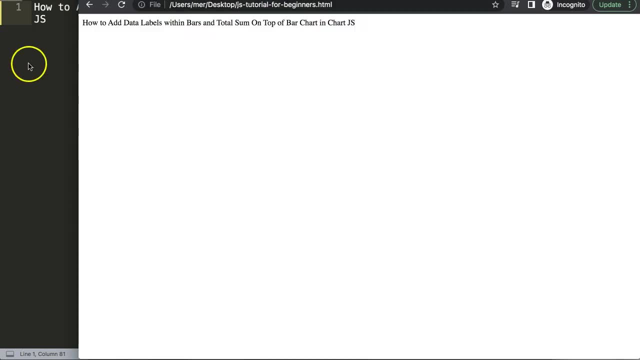 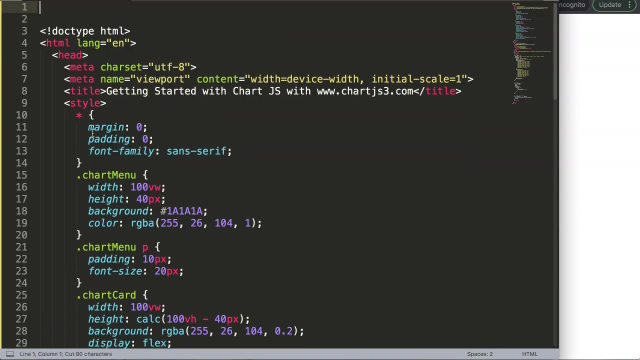 Scroll down and then eventually copy this entire chunk of code here, And if you want to understand what this code does, make sure you watch this video here. That explains it all. So then what I will do is I'll just paste this all in there, and once I did that, what I want to do here is move this title within the document here. 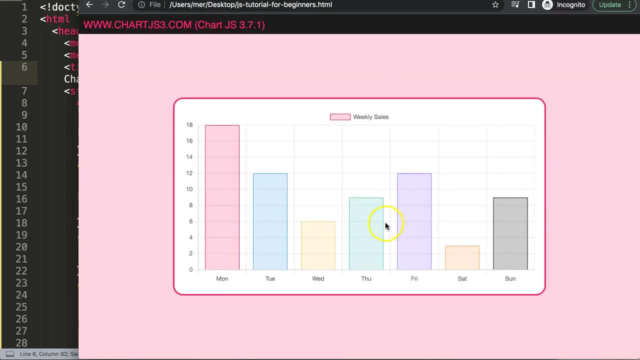 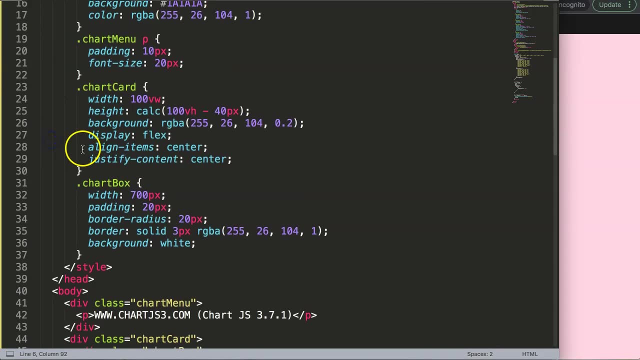 Save that and refresh. Alright, so now I have a bar chart, but what I need to have here is a stacked bar chart, because every individual bar should have a value or data label. so let's start to do that. So I'm going to just duplicate the data set. 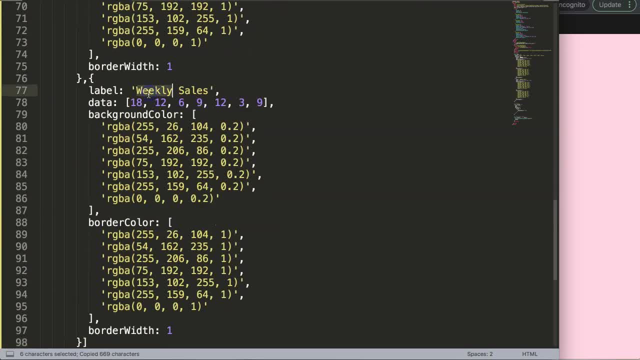 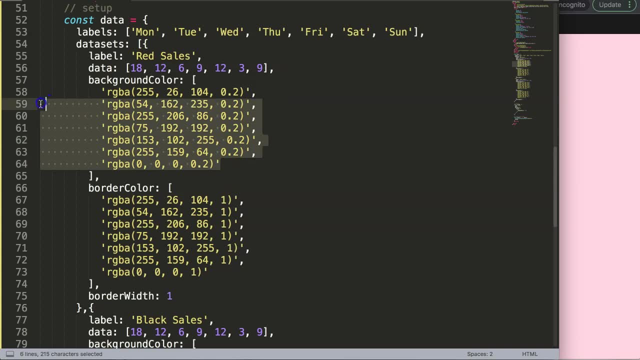 Copy that, Paste that in there, and then what I will say here, this will be the black cells, and here we have the red cells. So to do this I need to have, of course, the color. so I'm going to remove every color except for the top, which is the red color. 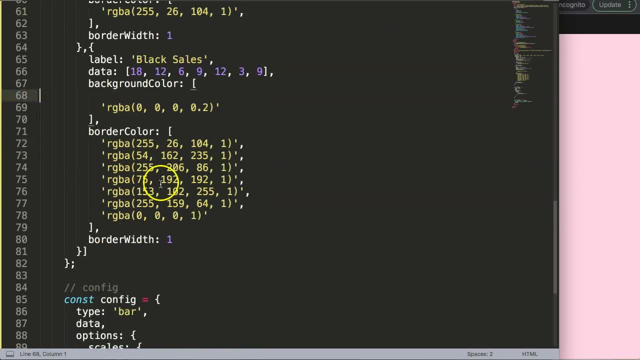 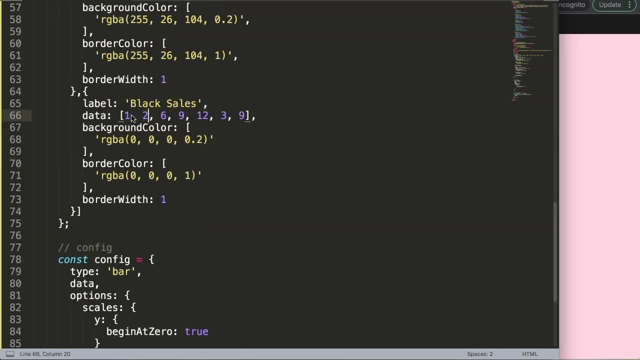 So we'll maintain the red color and here exactly the opposite, the bottom, which is a black color. Put it in there, Alright. to make sure it is clear, I'm going to renumber them all by a one to seven. So that's five, six and seven. so we can easily see the example. 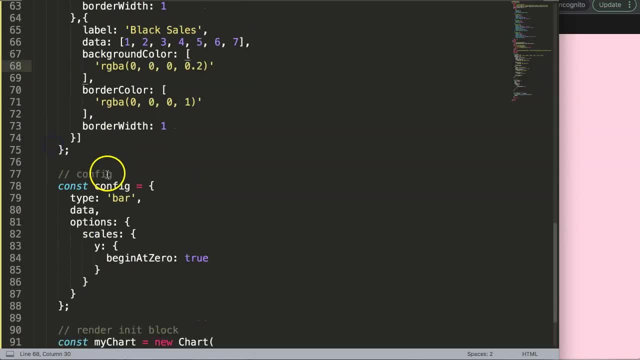 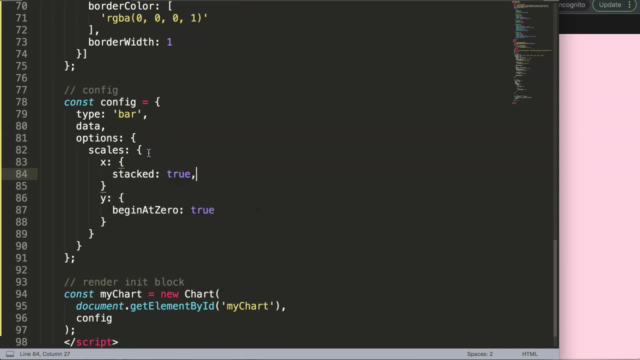 If I save this now and refresh here. right now it's not yet stacked, so we're going to activate the stack here. So we're going to on the scales we will say stacked equals true, and here stacked equals true, comma, and then make sure here I spell comma, or else we get an error. 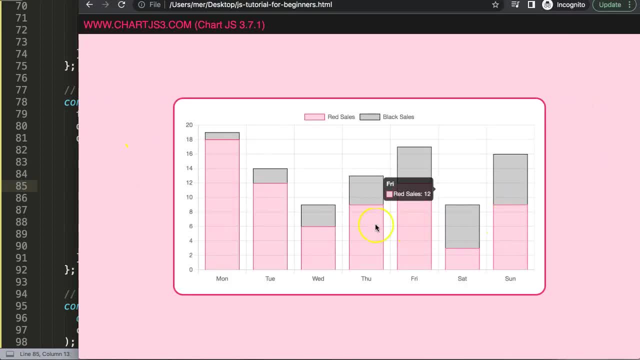 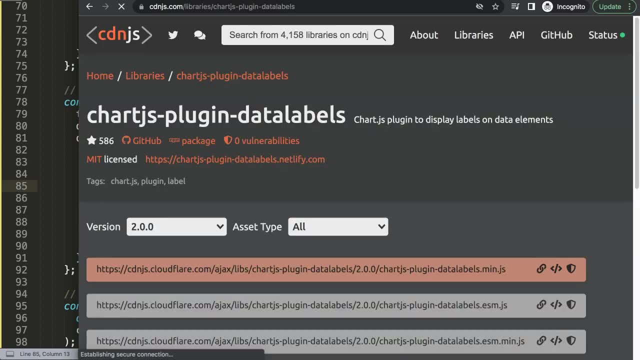 Save that refresh. So there we are. So now we have this. What we're going to do now is we're going to use the data labels plugin. To get the data labels plugin, you can go just to CDNJScom and search for the specific plugin, which is called the ChartJS plugin: data labels. 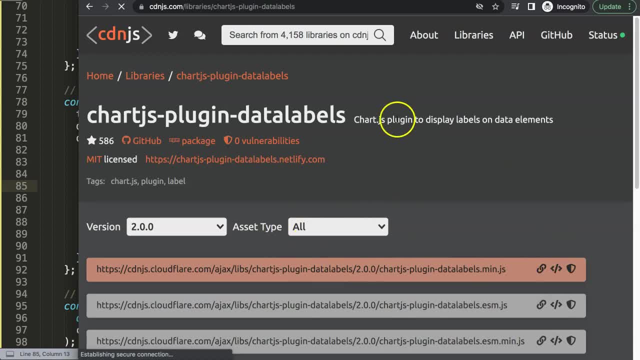 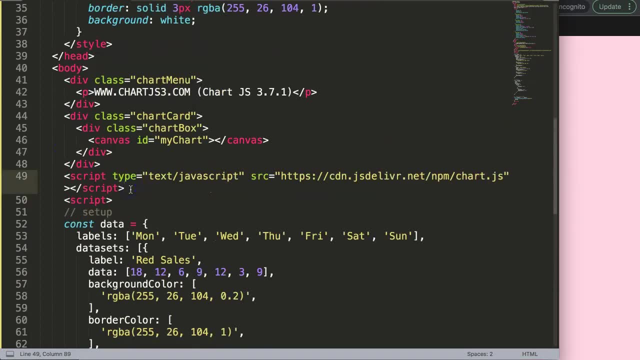 So I'm going to copy this and then you can click on this one here to copy the entire code, the tag in itself. So then I'm going to scroll up here on top and then I will paste this below the ChartJS library: Why? 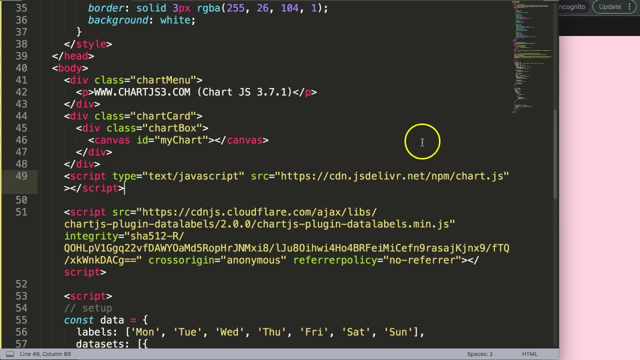 The ChartJS library needs to load first, because this plugin is basically an addon for ChartJS, meaning it has dependencies. that needs to be load first in the chartjs library and then this will work properly. so if I save this, it is not done yet let's scroll. 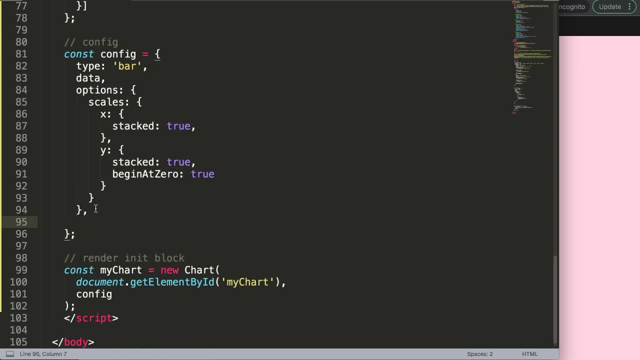 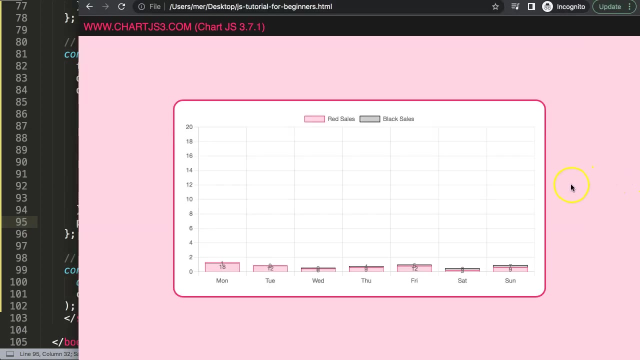 down here because we need to register or activate the plugin. so I put a comma here just within the options, as you can see. then I'm going to say here plugins and I'm going to say here chart data labels. if I save this refresh, there we are. it just took a second to load. now we have this. here is the next challenge is. 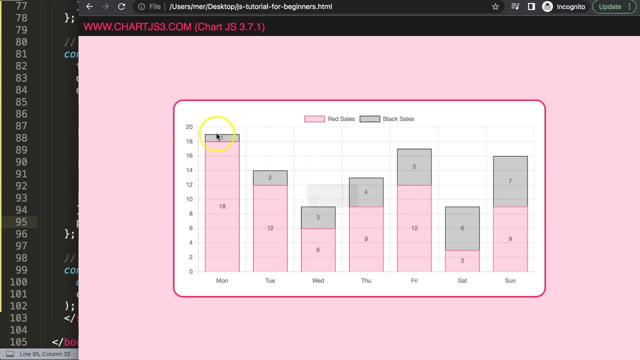 eventually is to put in the value on top here. this is not possible with the plugin data labels. or let me explain: you can move this up to the very top, but the problem is, when you move this one to the top, there's none within here, so this: 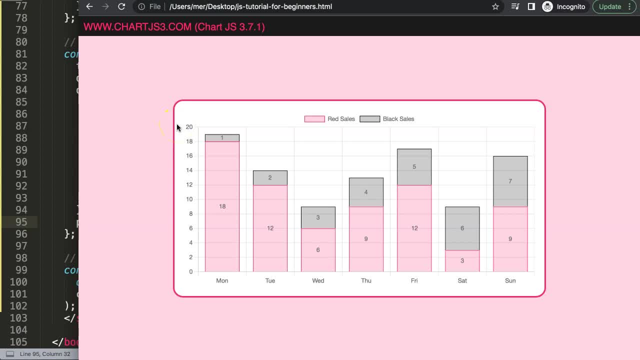 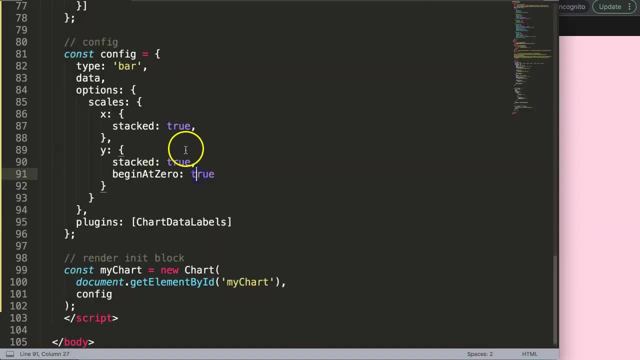 means we're going to need something else, and what I will do is I'm going to create a custom plugin, we're going to make our own plugin and put in here the total sum of here above. so let's start to work on that. so, the first thing, what we need to 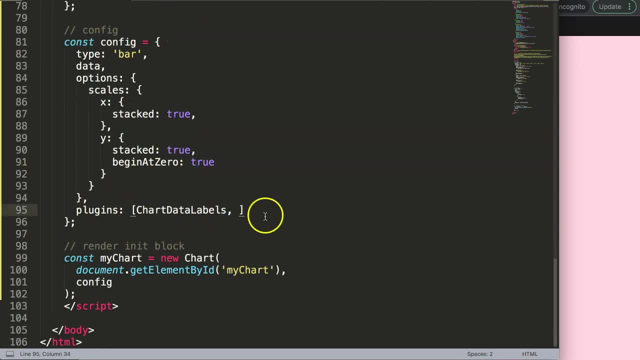 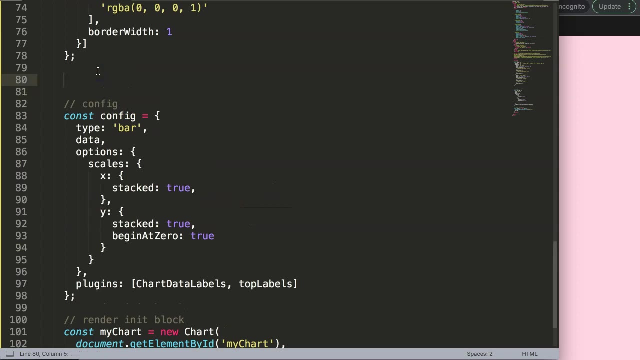 is to add up another plugin. to add up another plugin, we're going to put in here comma, because this is basically an array with an object, and then you're going to say here: well, just for the sake of it, you could say your top labels, that's basically what you want, it's a top label, and then enter, enter and in. 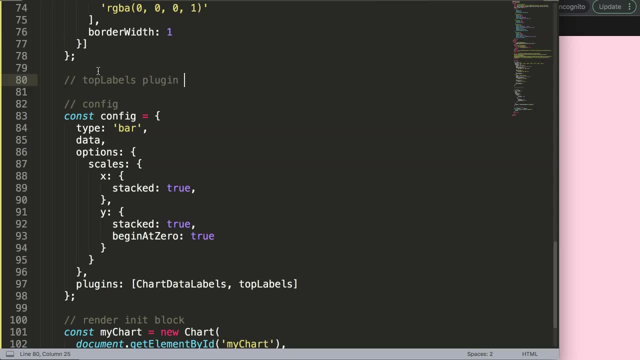 here we're going to say: here I'll just say this will be the top label plugin block. and I'm going to say: constant top labels equal, let's say, your ID equal to top label. and then what I'm going to say here is the drawing time. so when are we going to draw the top label? well, in our case, I. 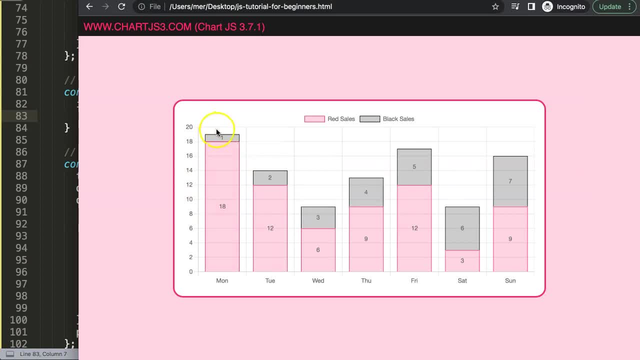 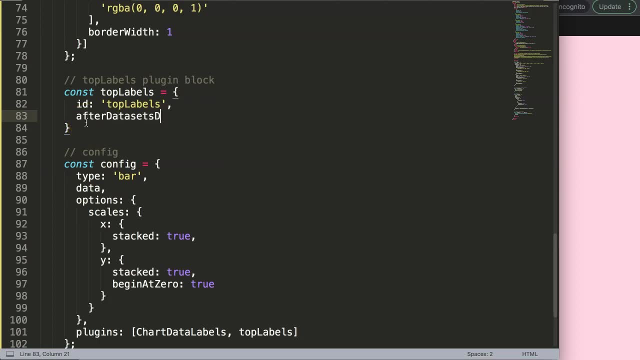 want to draw that after the data sets has been drawn, so it will be on top here and then it should be more than sufficient. so we're going to say here, after data sets draw, then we're going to draw this or activate this, this plugin. so then here we're going to have charts, we have your arguments. 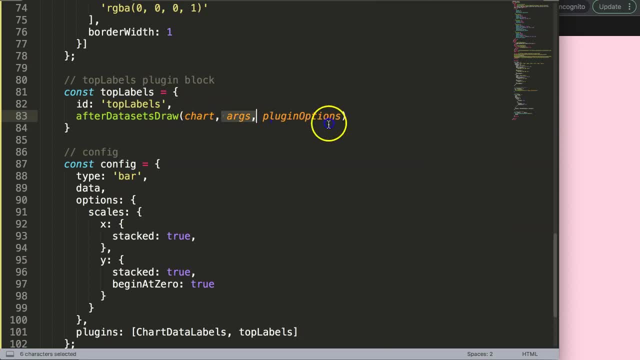 and then plug-in options, although the last two won't be used because these are directly connected with this. we won't be using that at all now, or at least not in this video. so then, what I'm going to do here is going to use object destructuring. 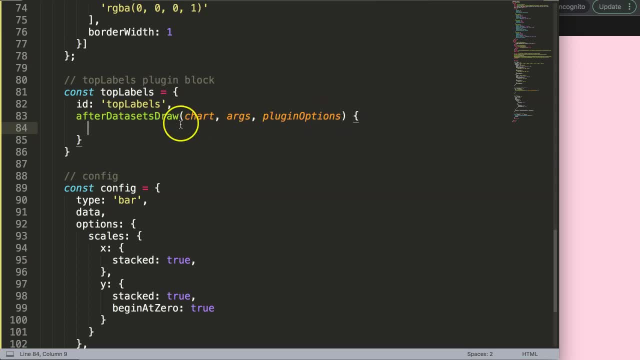 because the chart here has multiple objects, because these are all objects and we need to have the specific items here. so what I'm going to do here is I'm going to say constant and we're going to say curly braces equals chart. so basically, what we do is we're going to say here, we're going to say here, we're going to 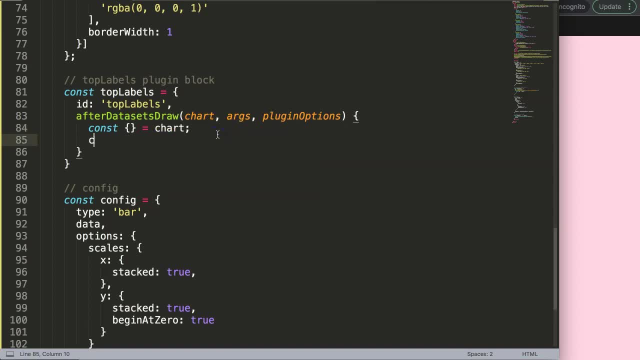 say: here we're going to do here is we want to draw, for example, something normally which we would have, that's a chart, dot, C, t, X, and this is such a long code if you have many different items, so that's too redundant and too complicated, so that's fine. I'm gonna say you now: yes, CTX. and this would basically mean I: 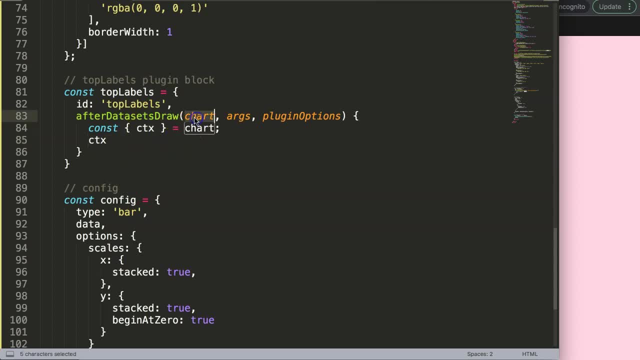 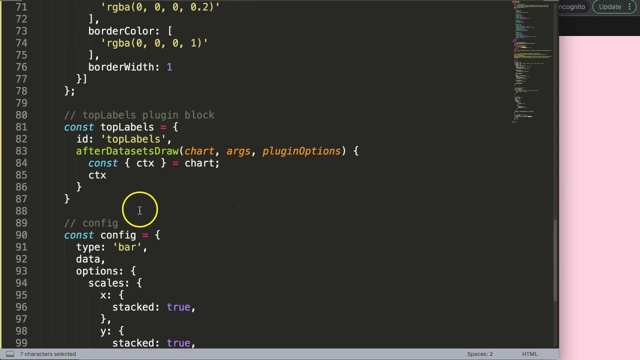 can now use CTX, and of course, there are so many more, because this here is the object of everything within our chart. so the one thing, what it is basically this one here with all the drawings in there. so so we have the C? TX and then the x, and then the z. so let's have a look at the background there. 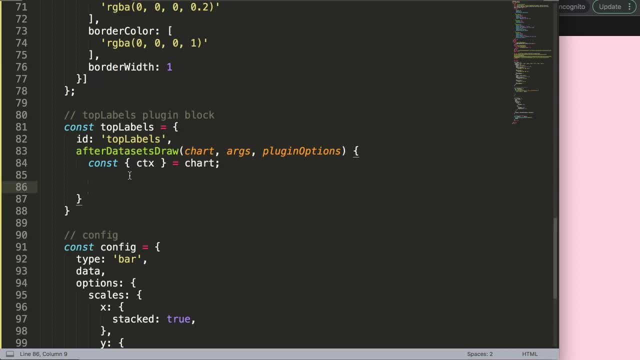 because this is what we do here right now. we have the x here now, and then the, which allows us to draw now within the canvas. so the next what we need is, besides the CTX, is the scales, and I need here the X and Y values. that. 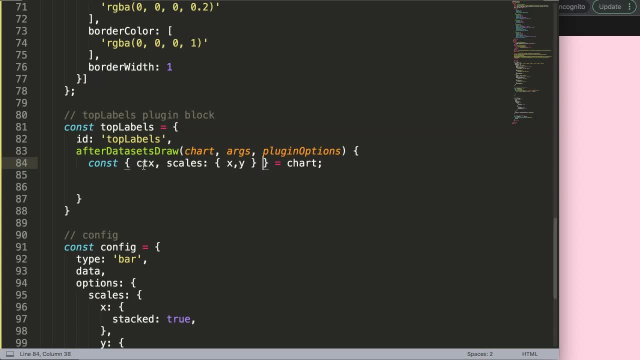 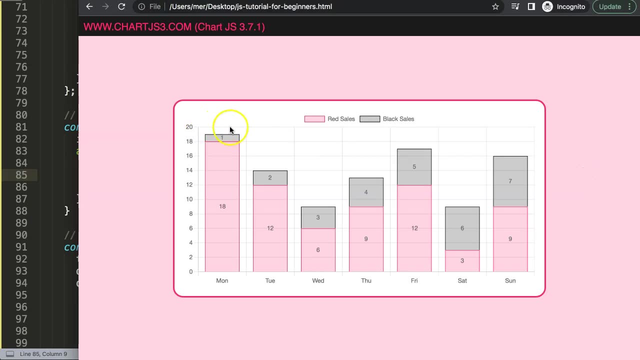 might be very useful for us, because we need to know the X and Y position of the items, because basically we want to make sure that's here at the very top. so we need to know the position in pixels here later on we're going to do that, Alright? so 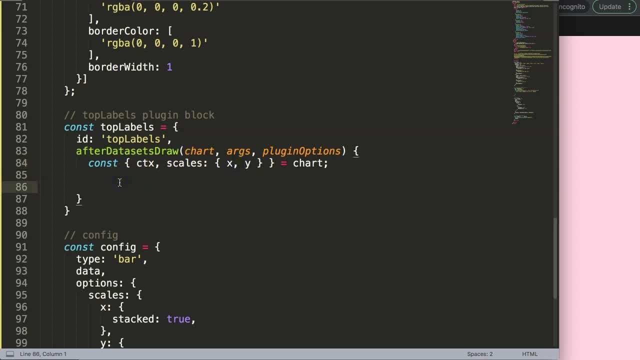 now we have the most important item for space here area, and what I want to do now is start to draw something. so let's draw something, and what I'm going to draw here now is just: first of all, we're going to CTX, and what I'm going to do here is: 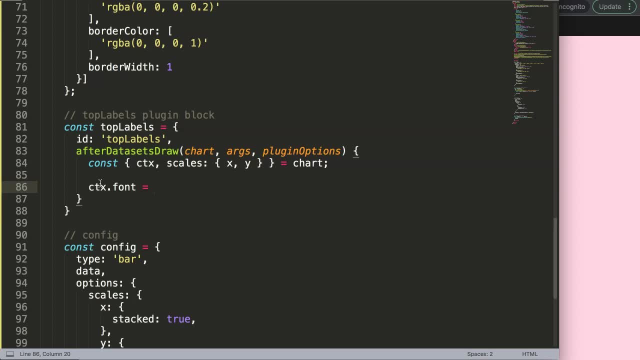 we're going to say here a font CTXfont, and I'm going to select a font style, font family of this. so for our case, I want to make this bold and I'm going to say here: this will be 12 pixels. make sure that is a string value. 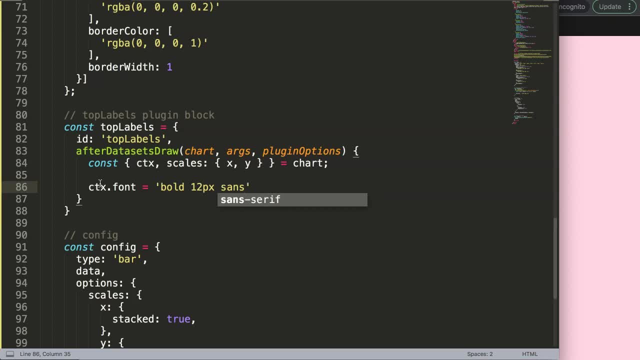 and then we say font family is sans-serif. once I have this, I want to say CTX dot and we can give it. here we will say fill style for the color. so in here we can say: here the color, what would be the color? for now I will just say blue. 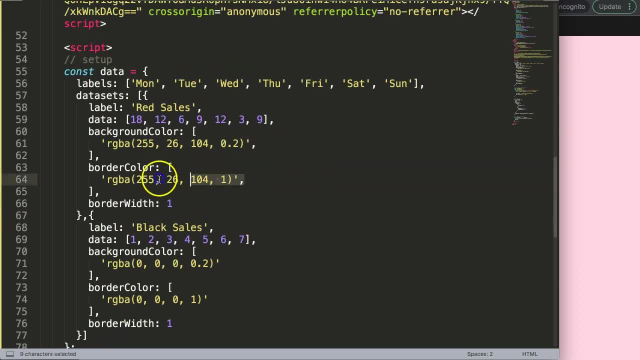 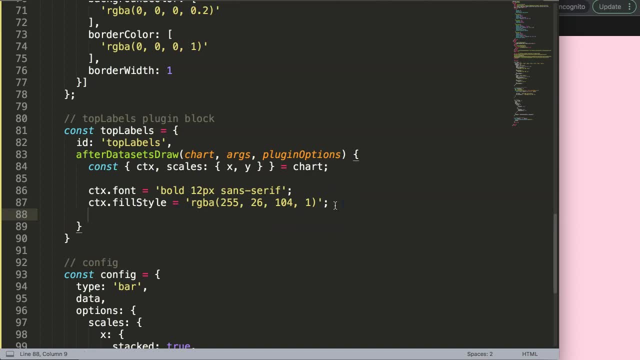 or well, let's get one of these colors here, let's grab this. later on I'm going to grab that color here, dynamically, set my column and once we did that, this we can do here. finally, CTX, dot fill text, meaning we're going to draw now the 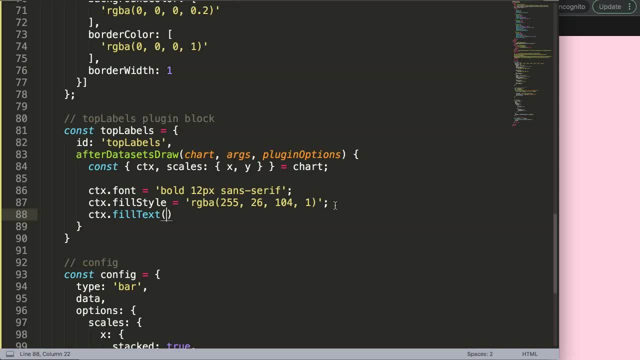 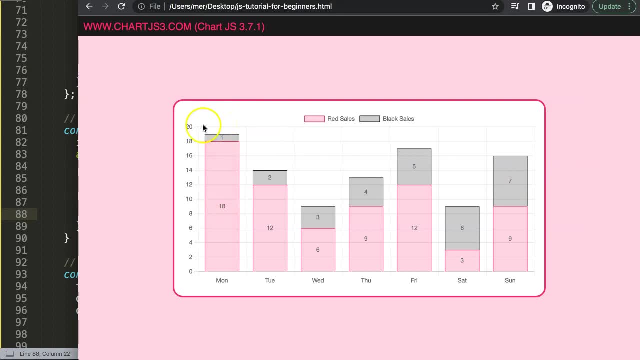 text and the two things. first of all, we have to put in here the text that you want to show. so what do we want to show? I want to show the sum of these two. so we have to work on that. that's a whole formula separate, so right now I'll just 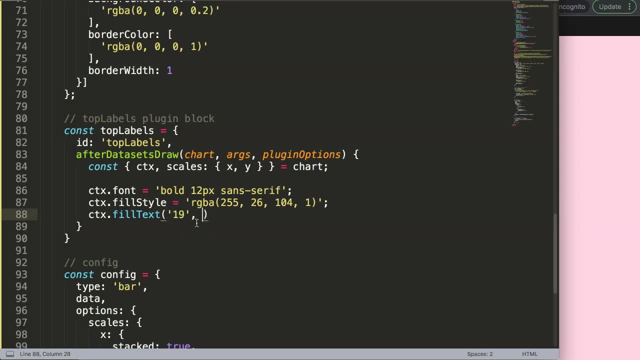 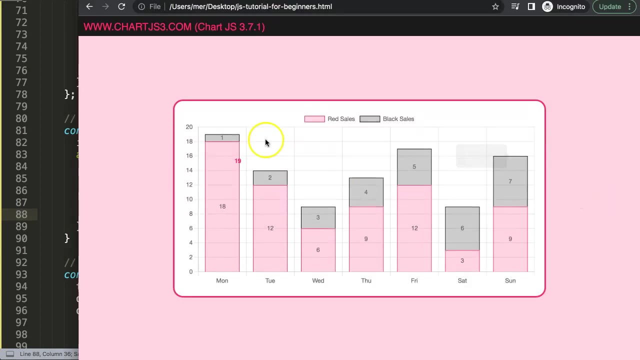 say here as a text, number 19 comma. this will be the X and Y position. so for this you still have to work on, but I'm going to put in here, let's say, 100 comma for the X and 100 for the Y position. if I save this, now refresh. you can see here. now we have something. 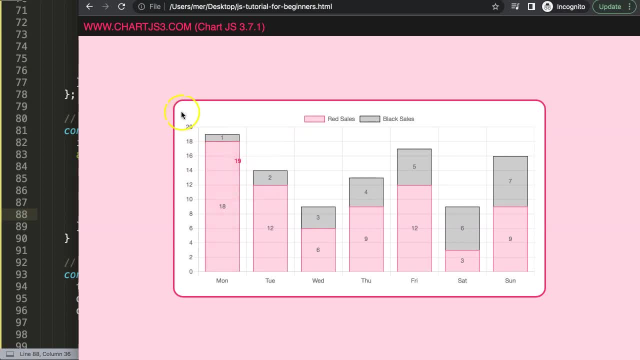 working, and this is apparently 100 by 100, 100 from this point. this is the corner here, and it goes 100 to the right and 100 down, or at least 100 pixels to the right and down. so what I want to do now, I want to make this specifically the 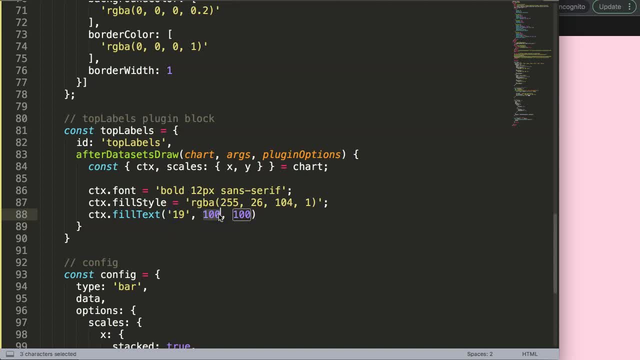 position, whatever we are on. so let's start to do that one. so I'm going to use a command here the X, which is referred to the scale, and then I'm going to say here, dot, they're going to get pixel for value, and then we'll put in here a 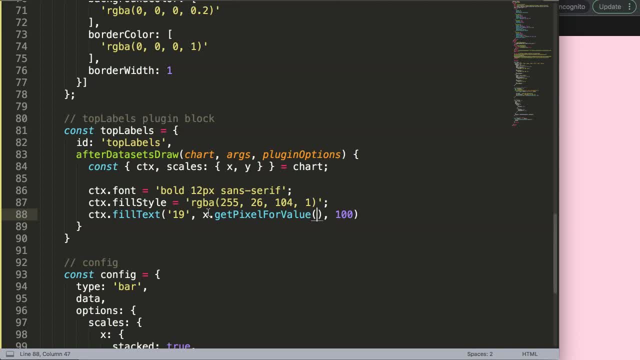 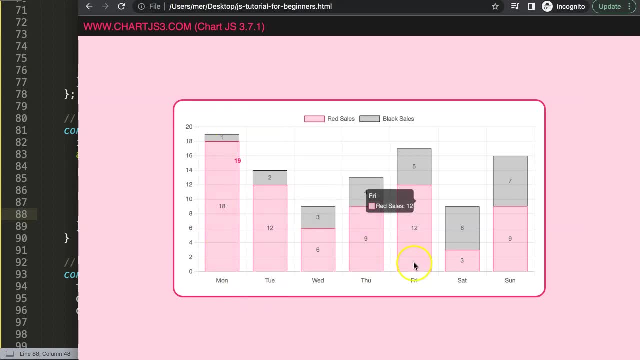 number, in this case our pixel for value, I would say here would be 0. and the reason why 0: because we're on the X scale, which is number 0, 1, 2, 3, 4, 5, 6. so I'm going to put this in here. if I save this now, you can see here. now it is. 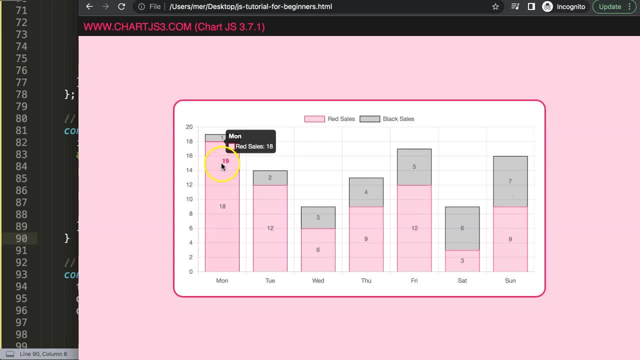 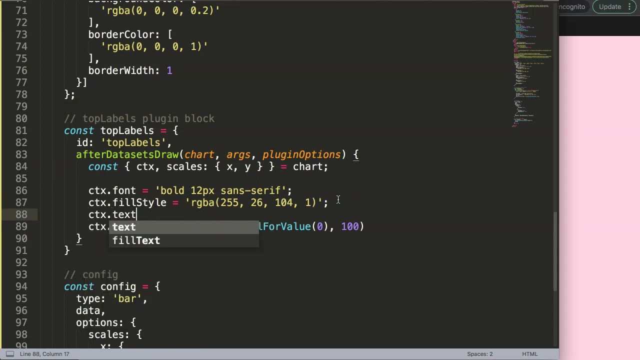 basically in the center, but it doesn't look like it. why? because we have the text align by default set on left, meaning all the left side will be ignored and starting this point. so let's convert the text align, or text alignment, to the center so the CTX dot text line with capital, a equals. 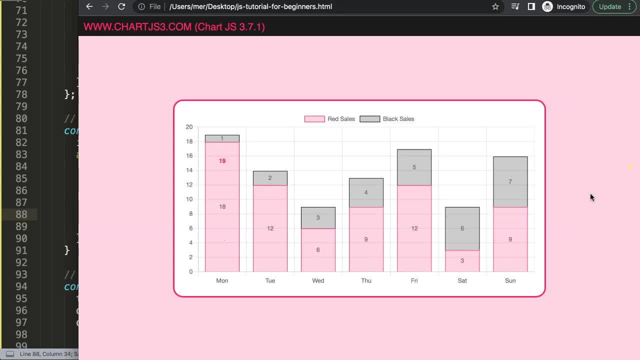 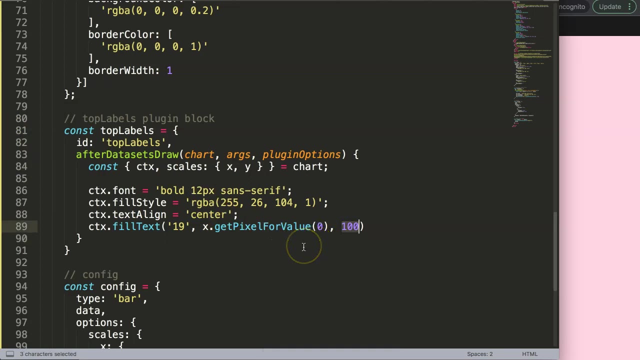 center. save this, refresh the area. so now we have that one. that is absolutely phenomenal. but of course we have now only D. Y prefer the X position. we still to have the y position, so for that we're going to use another command, because the y position here. 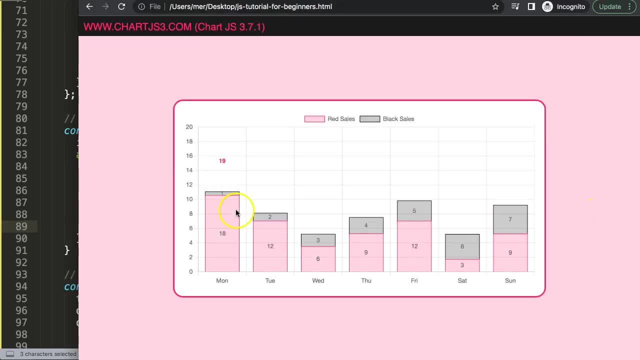 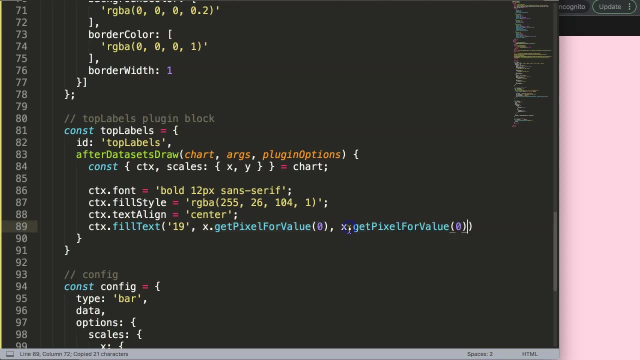 will be eventually dynamic, because we have this movement here, as you can see here, and right now you can see here, it doesn't move because it's static. so if you would do this, maybe you would say: all right, we just copy this and do this and then we just say: here, number 19, let's save that. 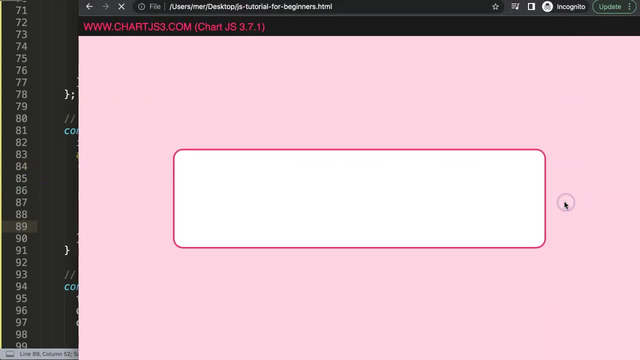 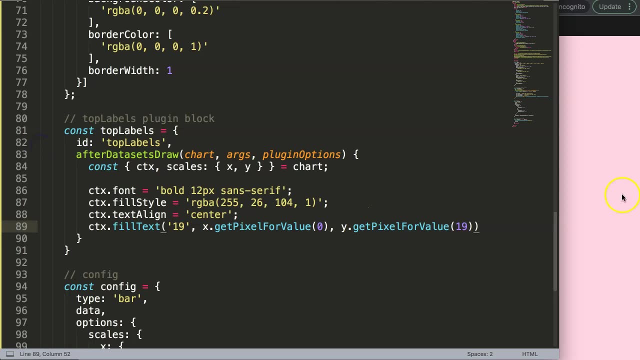 oh, of course not like. that must be white. this will be also static. i don't like the staticness of the static effect here. so what? what we want is this dynamic running effect, so let's start to do that one. so i'm going to say here: charge. so this is a built-in command in chart js, so the chart dot. 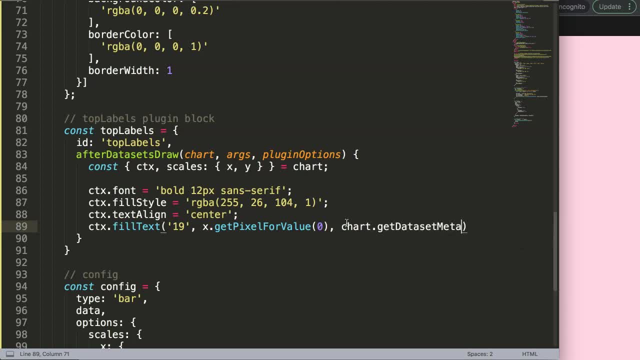 get data set meta, and then we're going to say it number, for now i'm just putting here number one, dot, and then we say here the data. basically, this is the method, would be the position, and number one and i say data, then we're going to get here the value. index would be zero, dot y. 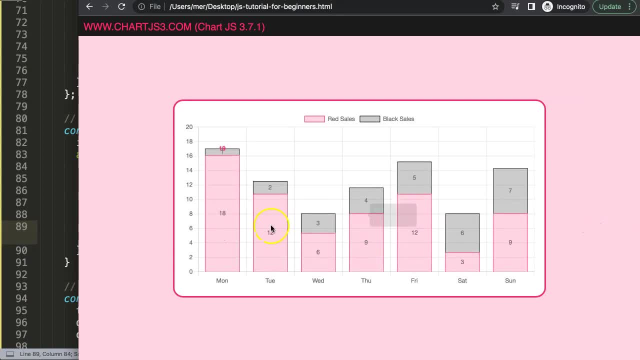 so if i save this, now refresh, you can see here. now we get the running effect. but of course, as you can see here, this is nice. but look, we have still one more issue, which is we need to push it up a little bit more, all right, so basically, this here calculates the pixel amount. so we're going. 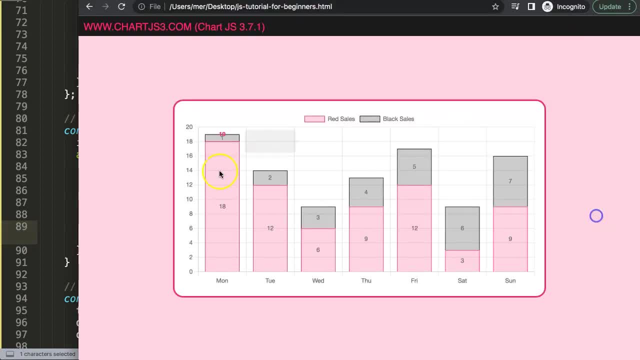 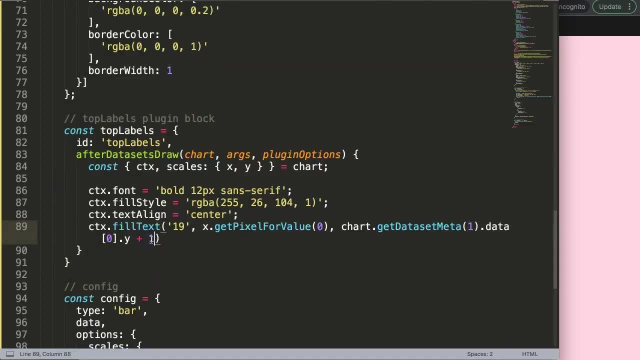 to do here is: it gets here the value, whatever the value is, but then convert it into a pixel amount and that's why we have the running effect and it works nicely. so now i'm going to just say plus- oh no, sorry, not plus, but minus: 10 pixels. y, y, minus and not plus. if you go plus, we're going down, because the top 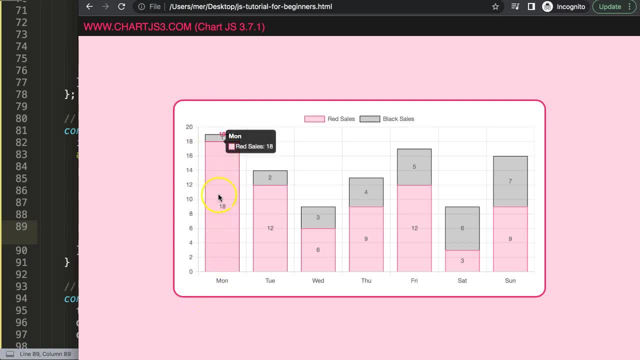 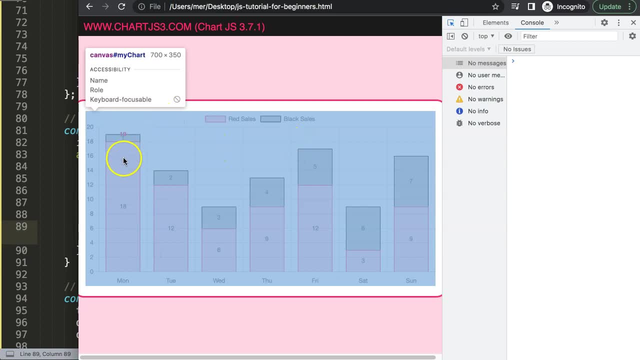 here is zero, down here is: whatever the height would be of this canvas which we can search here. let's do this. you can see the height is 350.. so if you go more down it means a higher value would be. or this is 350, halfway here, 100, 175, and up here is zero. so i need to go and reduce the amount. 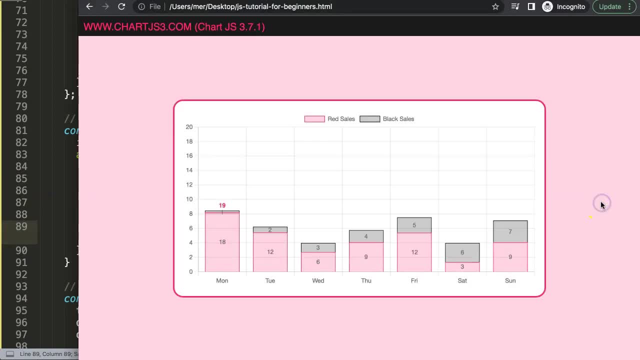 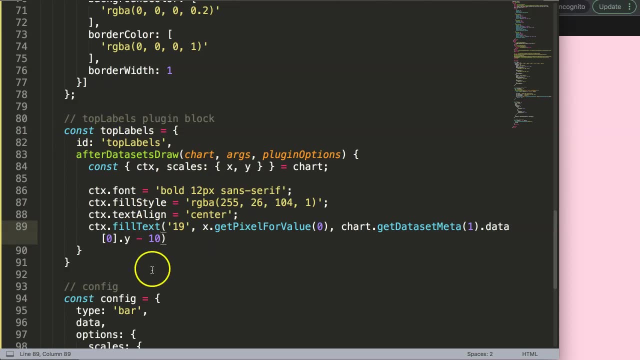 whatever we have here by minus 10. if i save that, refresh there, we are all right. so we have this now and we're very close to it, because what we need to do now is start to loop through this entire item. so what we're going to do here now is: let's see. 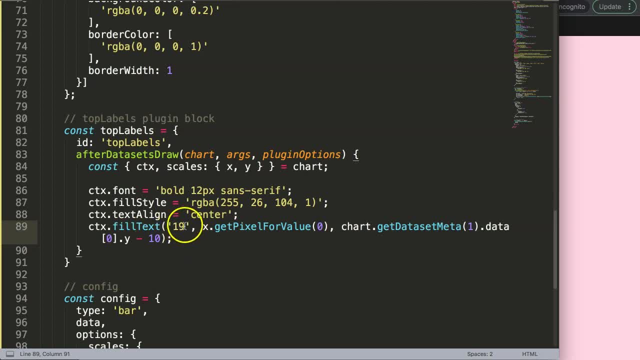 uh, we have this, but now let's start to loop, and of course, this is hard coded. so far, i don't want that, and this one here is also hard coded, and this one can maintain, so that's fine, this doesn't matter so much. so what i'm going to do now is: let's see here. what we have to do here is: 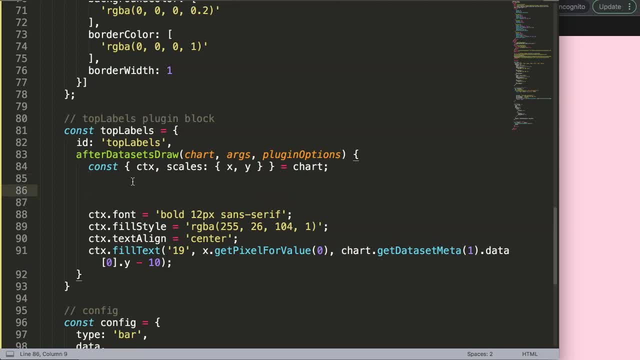 we're going to enter, enter here, and then i'm going to create here a chart, dot, data, dot, data sets, index, zero, and then we stay here, a dot, data, dot for each. basically, what i want to do here is i want to loop to rather what exactly one? i want to loop to every individual data point. 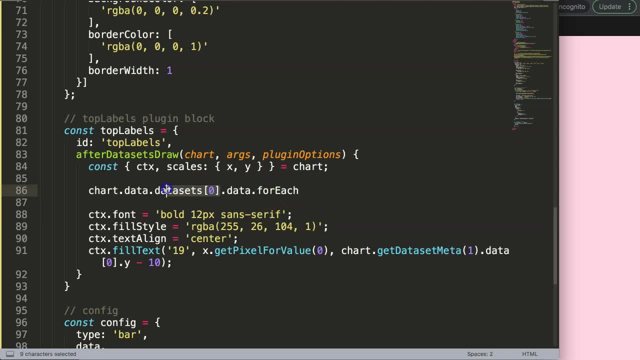 so we're going to do that one and i'm going to show you. you might say well why we do this? because we will be missing data set number one. don't worry, i will have it on a trick for that that will loop through both data sets, but first of all i need to know how many times we loop to. 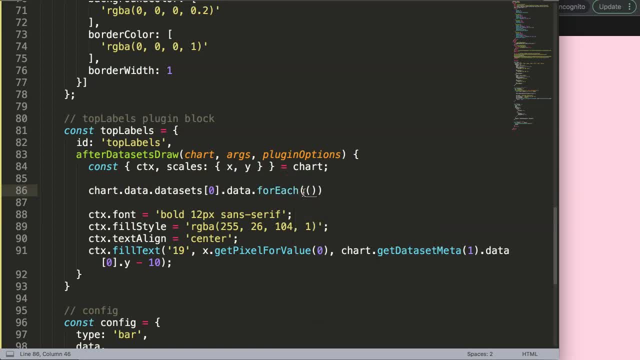 so i have like this here already. so then in here, what i want is: i want to say your data point, so this will be our data point and the data point and, of course, our index. all right, once we did that, we can have here a function error expression, because it's a callback functionality here. 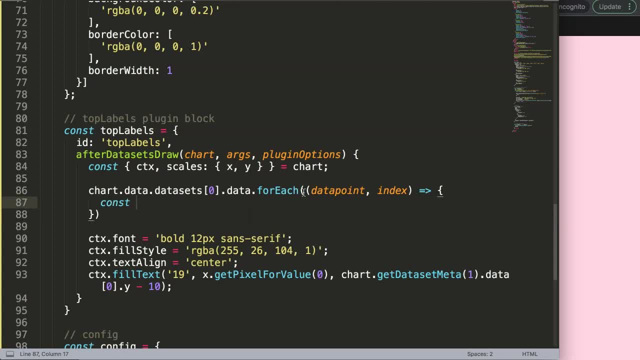 and i'm going to say constant and i'm going to say here: this will be our data set array. what i really need- well, let's say equal this and make this an array- what i truly need is to loop through all these items here individually and then push them into an array. 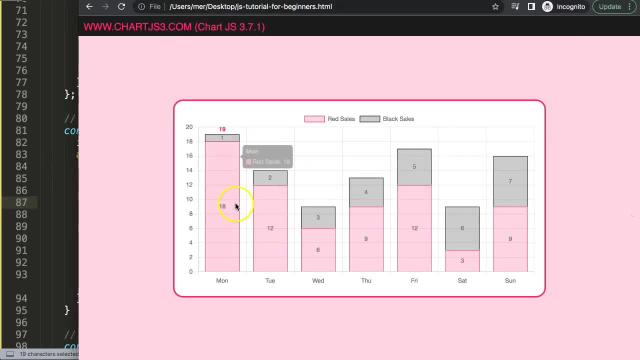 however, every array is specifically for that data set. those who are matching with the data point here: 1 and 19, or 1 and 8, 18, sorry, 2 and 12, 3 and 6, etc. etc. this needs to be connected. i don't. 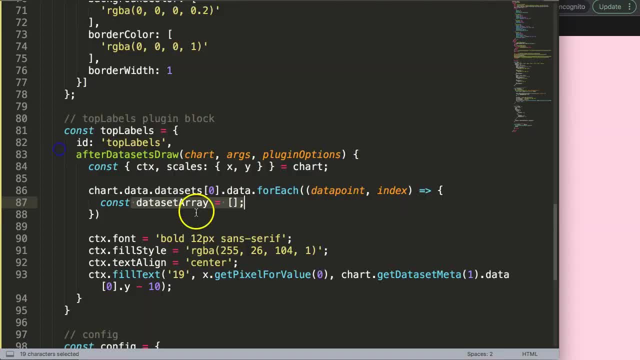 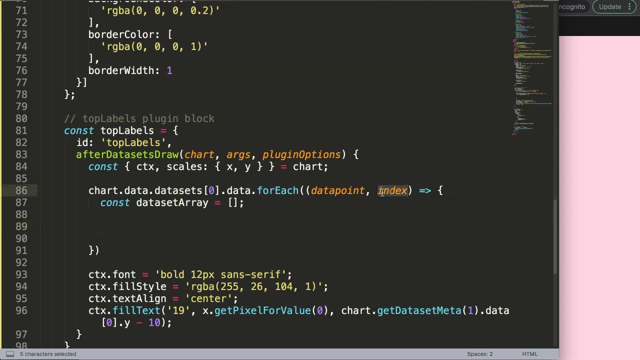 want them all together like this, because we cannot have the sum here. so this is very important. so once i did this, i have this here. then what i want to do is i'm going to put it here, enter, so within loop, because we have the index here, one from zero to six. this is very important. 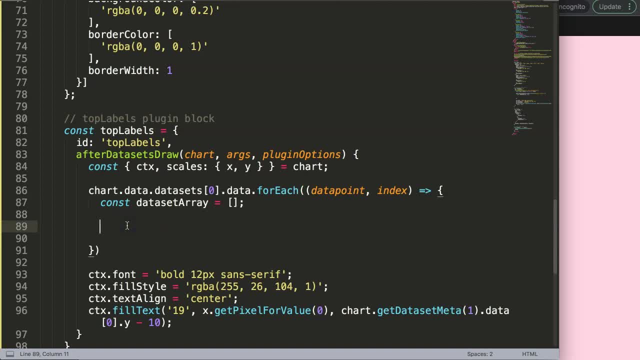 we can start to move on. so what I want now is the following: I'm going to say here: chart, dot, data, dot, data sets. there's a dot for each, and what this truly is is the following: I want to have here again: same for a for each loop, but 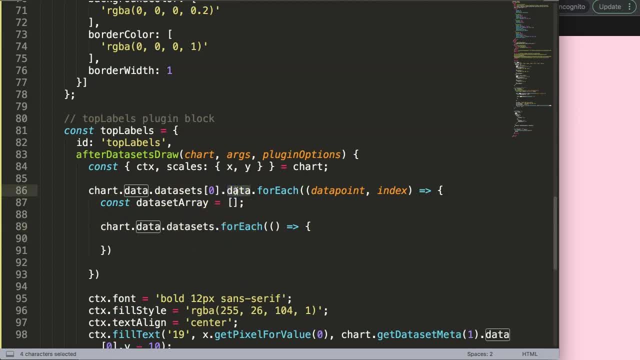 this one here is for the data set, so this one was specifically for the seven items or data points. this one is for each data set, so I'm going to give data set comma. well, I don't want to have your index, because if I will have index here, 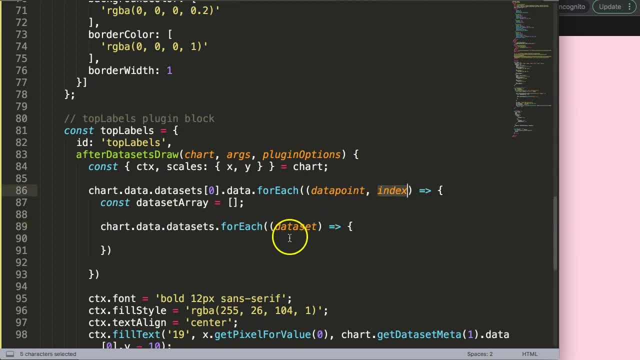 I will have a conflict with this, because I need this value here. so here we don't need to put in a comma index, or else we have one and two and this will be- or sorry, zero and one, and this will be zero till six, because we have six or seven. 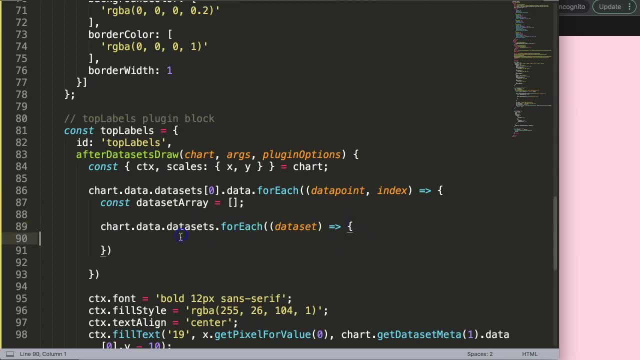 data points, and we only have two data sets here. so that's why we don't do that, or else we will destroy the precious value of this one here. anyway, we have this here. what I want to do now is I want to say here the following: all I need to do here is basically this. I'm going to copy this: 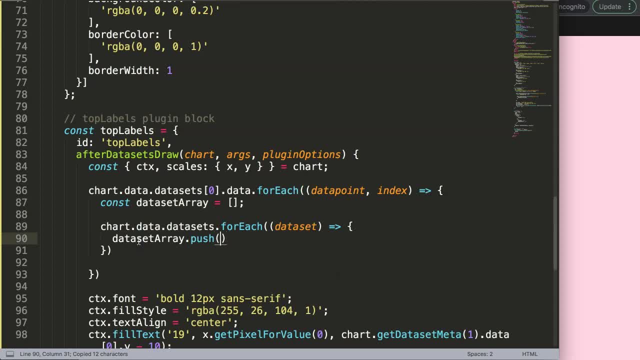 the words are: you thought: push what I'm on the dot, push here in this data set. you're going to say yet dot, beta and data and to say: here we can put in here index, all right, so once we have that, we should have now the numbers. 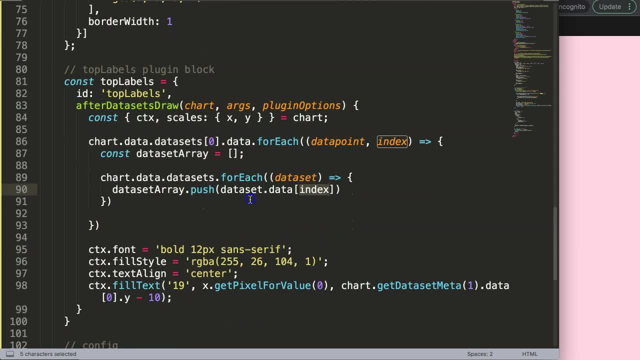 pushing them for each of them. so this is very important. so the index would be basically zero, one, two, three, four, five, six, seven, or one two, six, but here, because we have two items, it will go then to data set, one, which is basically this: here we first get this one in this data set and then that. 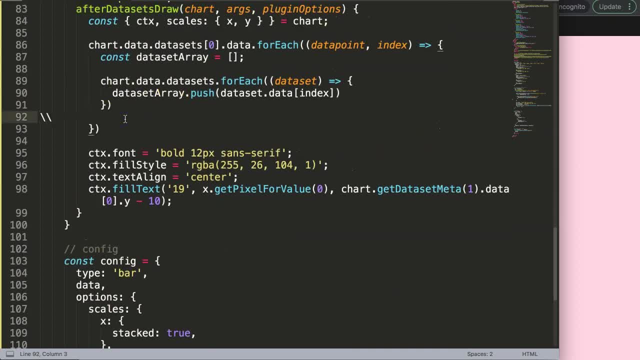 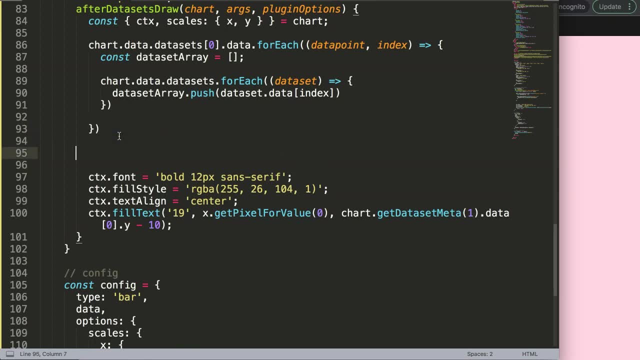 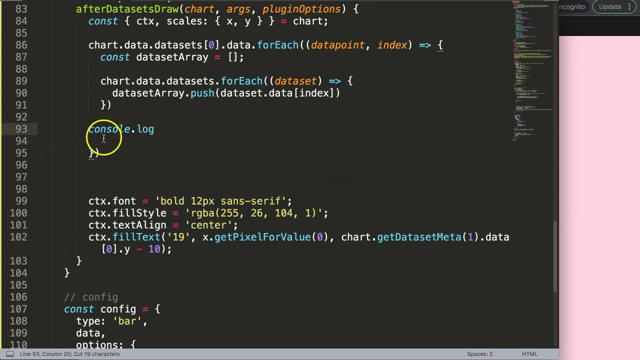 one. all right, to make sure that this is correct. what i want to do here now is, of course, a console block. uh, let's see, here we can do the console lock, maybe even in here, say here console. oh sorry, i cannot do that in there because you have to do it within the loop. 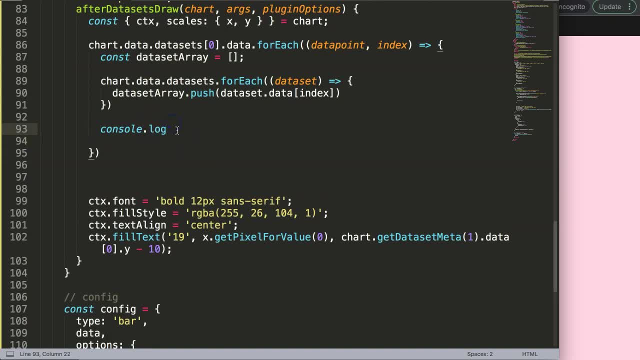 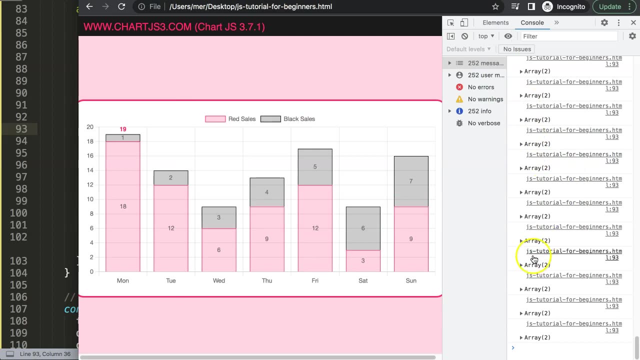 without the loop, it will be in conflict. so why? because in the loop, individually for that one, or else outside the loop, you only get the last one, because it overrules itself of overwrites itself. so then let's save that. refresh, all right, we see nothing yet, but we get an array here. we get many. 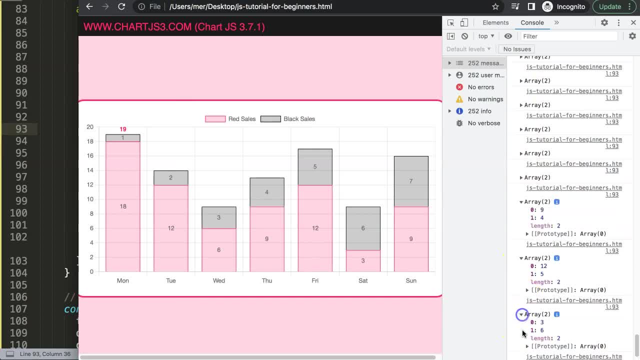 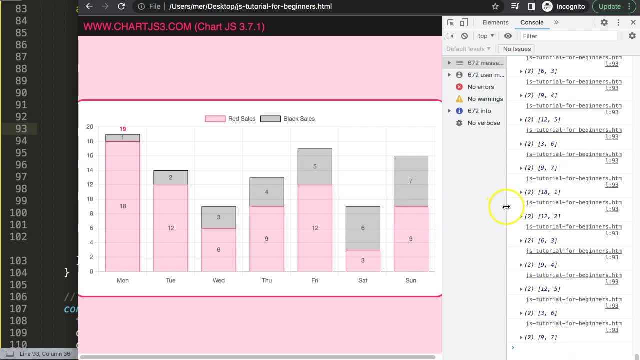 information here. all right, you can see here. all of these arrays are directly matched: seven, nine, and if i loop over, if i move over it, it will trigger it again, but that's all right. so you can see all the information here: eight, eighteen plus one, twelve plus two, which is this: 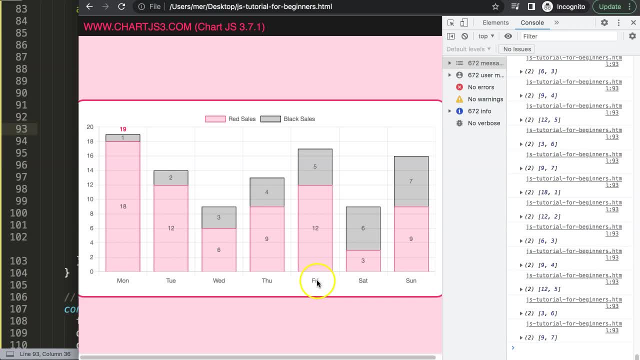 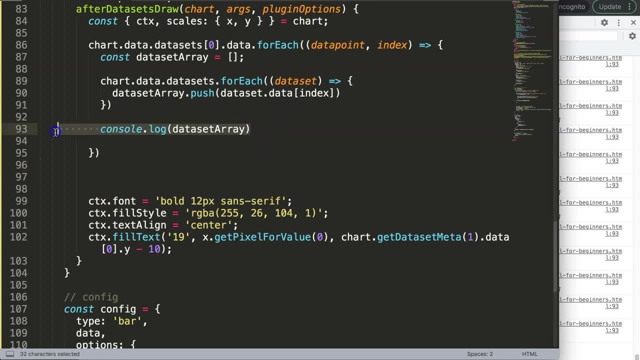 one tuesday, six plus three, uh, nine plus four, et cetera, et cetera. so this is already a working model, so now we're getting very, very close to it. of course, what i want to do next is: i need to have the sum of it. i don't want to. 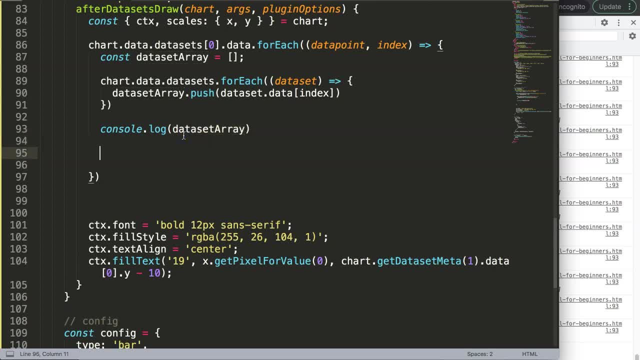 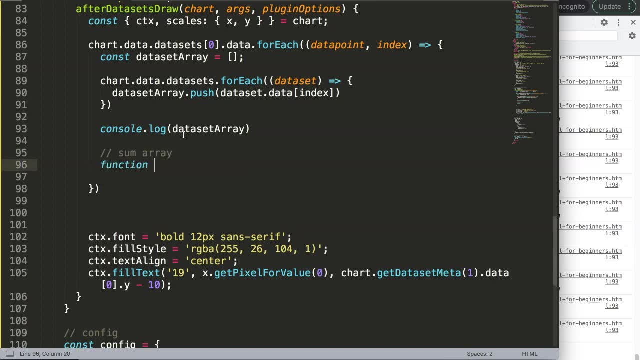 have this array, only i want to have the total sum of this. so let's start to work on the total sum. let's say a sum array and then what i'm going to say here- function. we're going to say here total sum, which is basically total comma values. 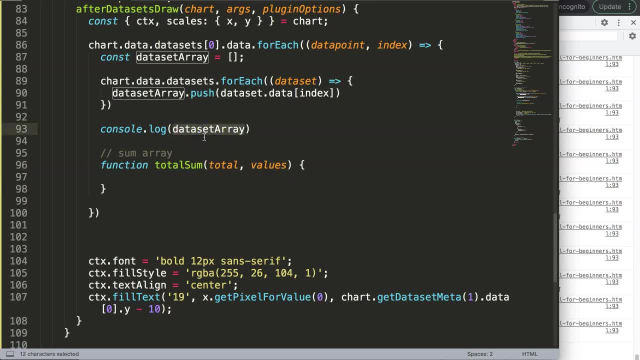 and what this really means is that we're going to grab later on this item and every individual value in this array is a value. we'll be plussing it or adding it up on each other or summing them together. so we say: you return the total plus values, all right, so this goes in here, and then we're going to say: 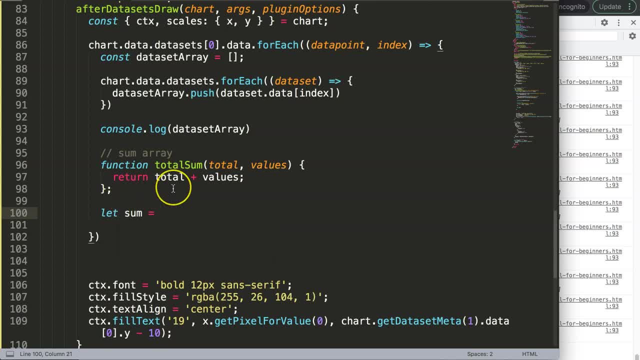 let sum equal, basically reach array. that's this array. we're going to sum this specific array and then we're going to say here: dot, uh, dot, reduce. that's the command over the method, and the reduce will be used with the total sum functionality. here, comma, our starting value will 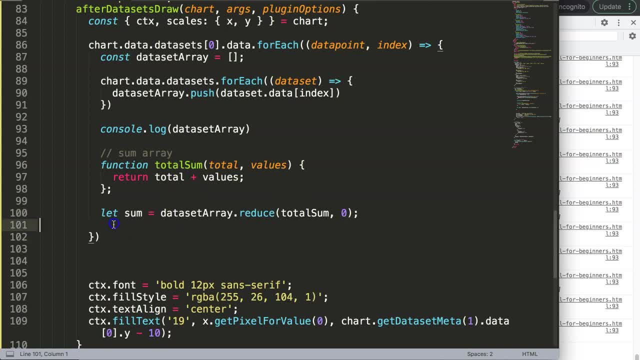 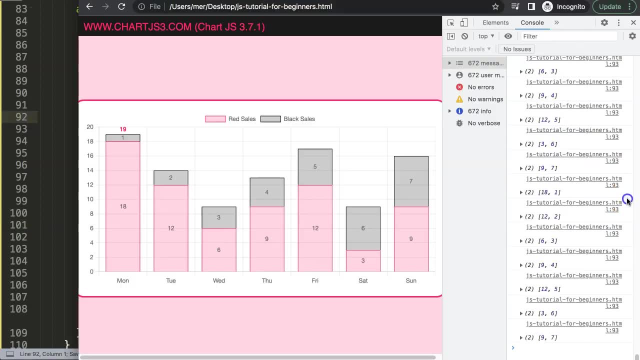 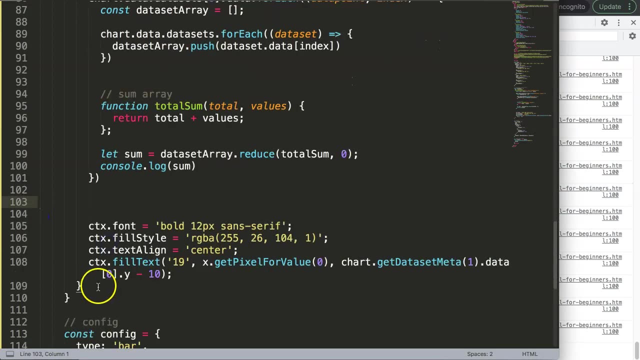 be zero. once we have this, you will see now if i have a console log sum which will have another value. save that refresh. all right, so we get now all the values here. you can see in 1914, etc. etc. all these values are showing. so now of course let's see here this item. we can cut this all on. 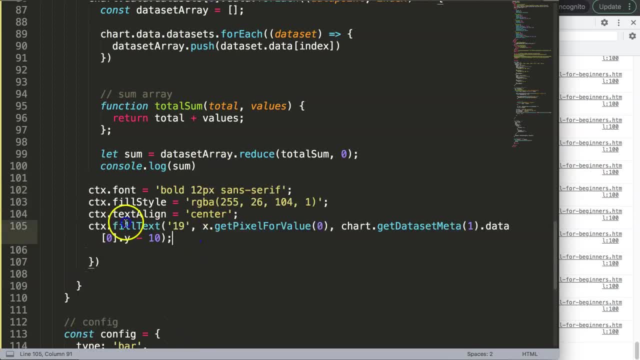 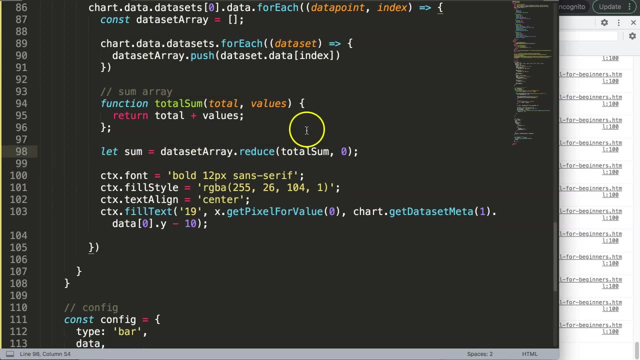 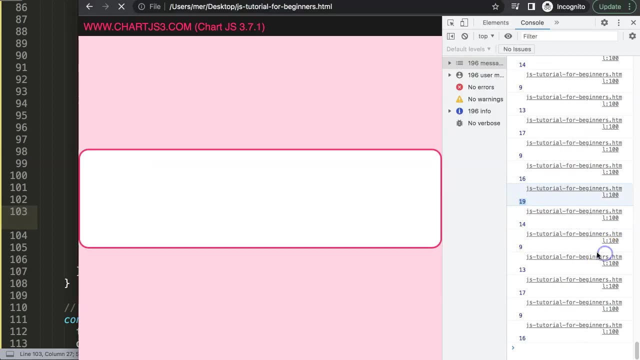 we have this, all nicely, put it in here, give it a proper indentation, all right. and then what i will do is i just remove this console log sum. but i'm going to grab this sum here, put it in there or as a variable, so it's a variable, not a string anymore. save that, refresh, all right. so now we have them. 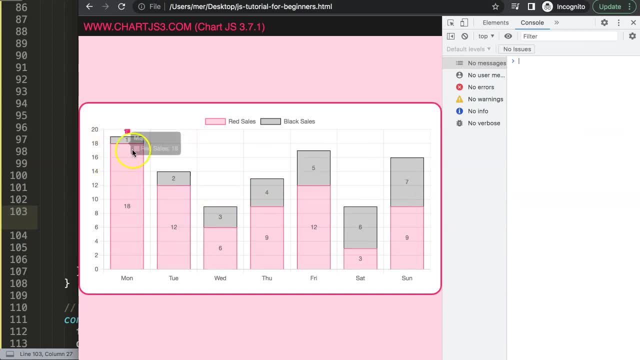 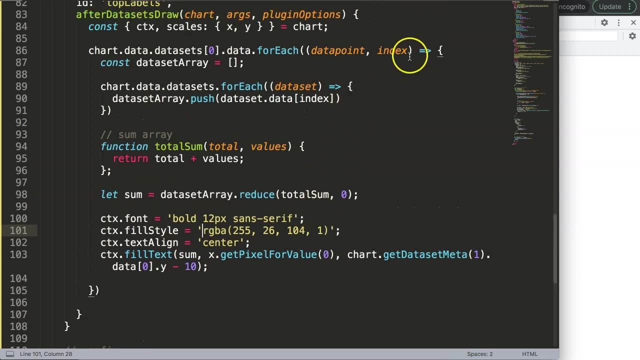 but you might notice one thing: it is looping on top of each other. so i don't want that. so what we're going to do here now is we have this and then we're going to do this, and then, of course, remember we have this index because we're still within our functionality and 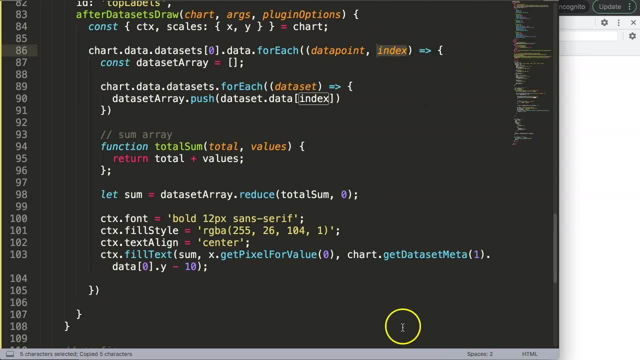 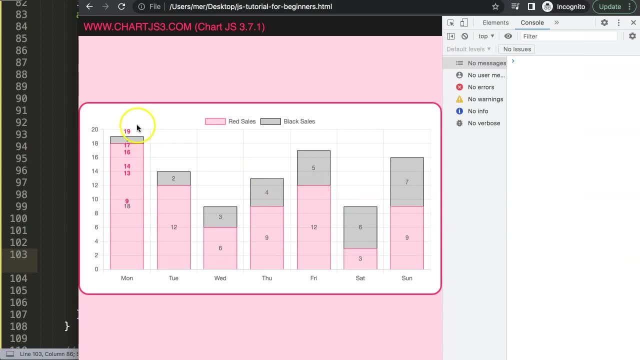 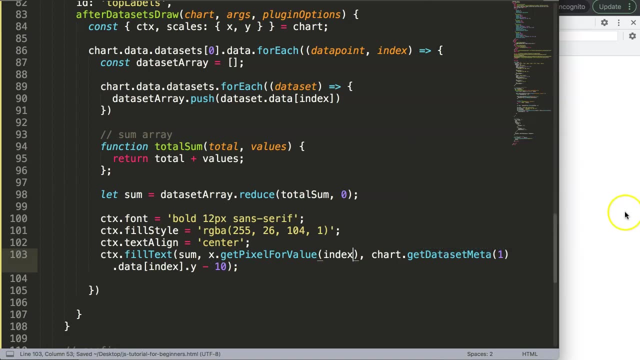 this index is still for us very important. so we're going to copy this and we're going to just put it in there and let's save that and refresh. let's see here, all right, now we get the height for the knee and then here we can probably get this one, the index, here as well, refresh. 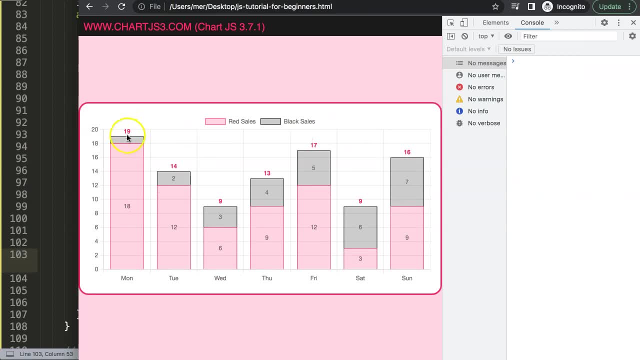 and there we are. so now we have this here. but you might say, hold on, look what happened here. if we are too high, what will happen? if we're too high, what will happen if we're too high, what will happen. so let me show you here: if you put here another two, save that refresh. so oh my goodness, we're. 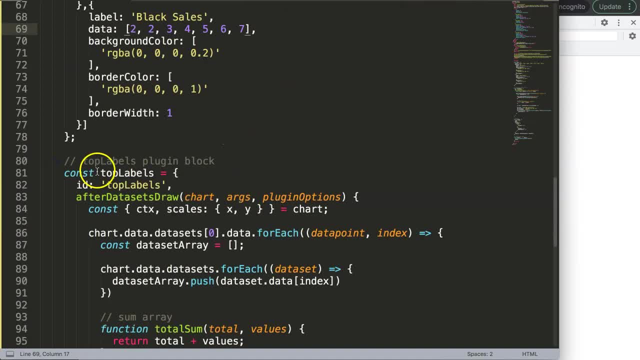 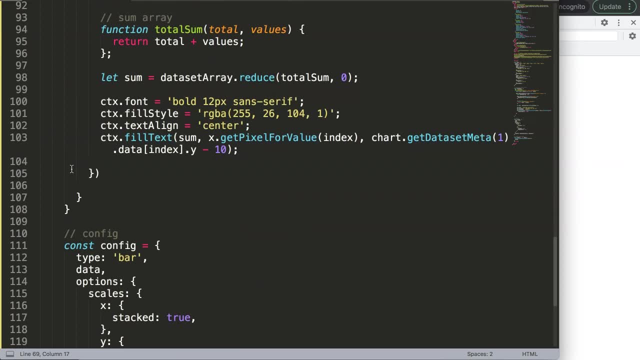 going to hit the legends here, and that's i'm very sensitive to that as well, so i would not want to accept that. so what we're going to do now is going to give this what we call a grace, uh, space, a space of grace period or grace. well, i guess a grace period would be not the right term, but a grace. 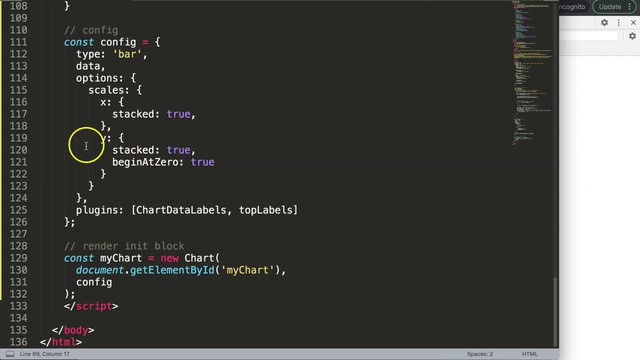 is the term for additional space to consider. so we're going to say, here on the y scale, put a comma and the grace amount will be. let's say: uh, let's put in five points, or maybe four points. save that refresh. there we are, and now we have some space here. we could even reduce that, depending on what. 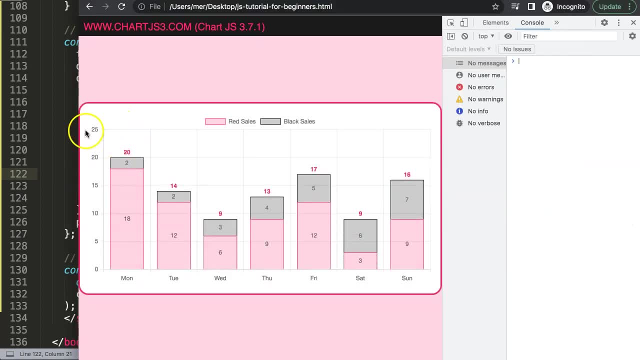 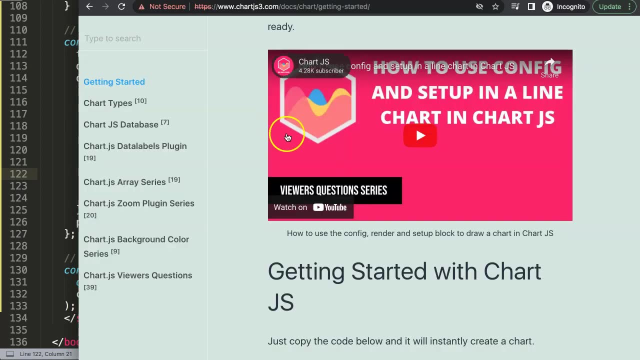 you want. there you are, apparently. we'll just calculate the brackets here. that's all right. so we have this here. if you might say, well, what about if i want to get the color? so let me show you something. so let's get these colors here that we had in here. we're going to grab these colors here. 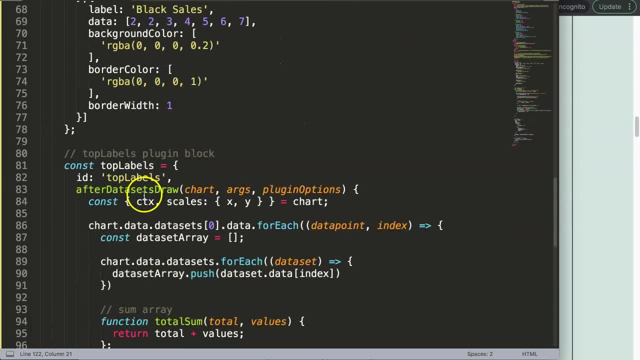 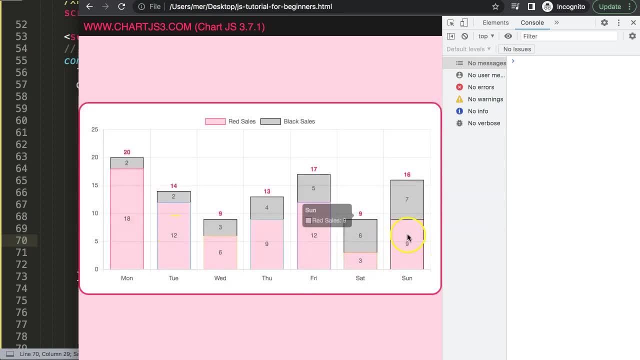 of the border color. i'm going to put it in the middle. and then i'm going to put it in the middle in one of our data sets. so we're going to say here: put that all in there, let's save that. go back here. now we have all of. 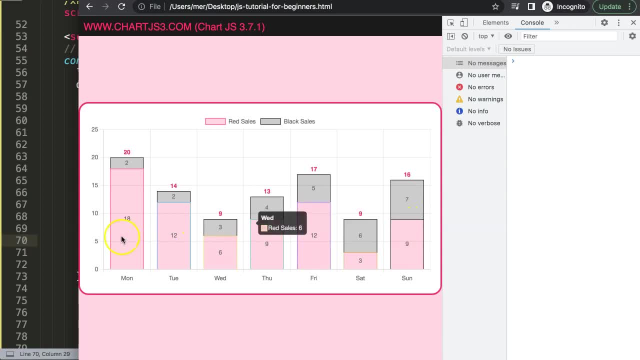 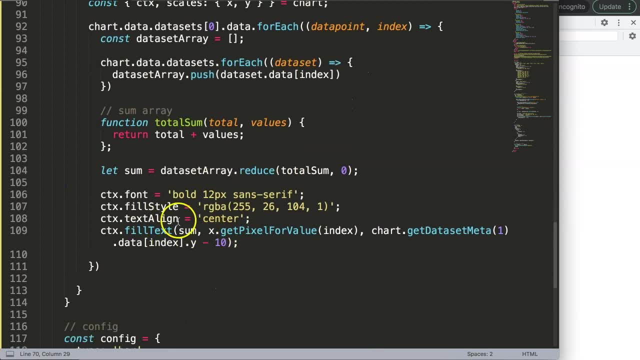 this the border color and the background color, i guess. and let's get this border color put it in here, so we have matching colors, all right. so how do we do that? well, what we have to do here is we have the rd color, and all i want to do here is now basically the following: it would say a chart. 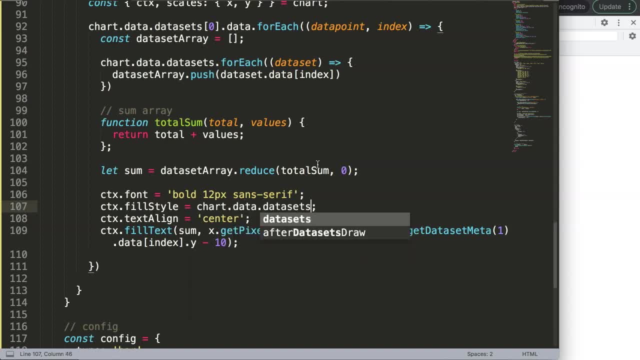 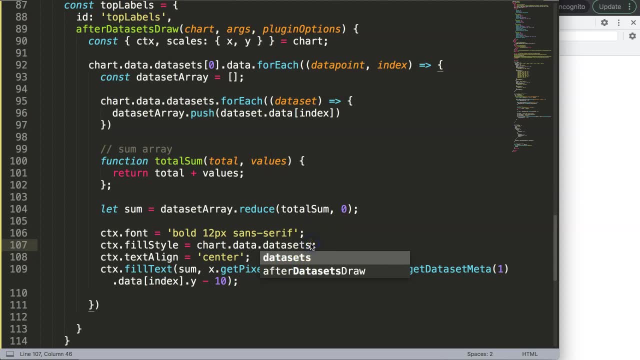 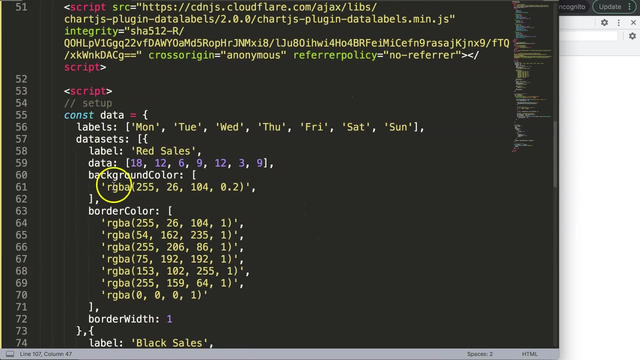 and we say dot data, dot data sets, and maybe we can even. i guess we could even do. can we do that? no, we cannot get the data here. that's not possible. i thought maybe the data point here was not possible. so we have to be specified individually and i'm going to say in the data sets what we're going to do here, the data. 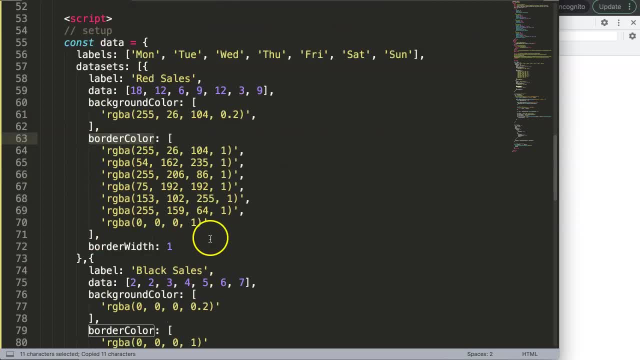 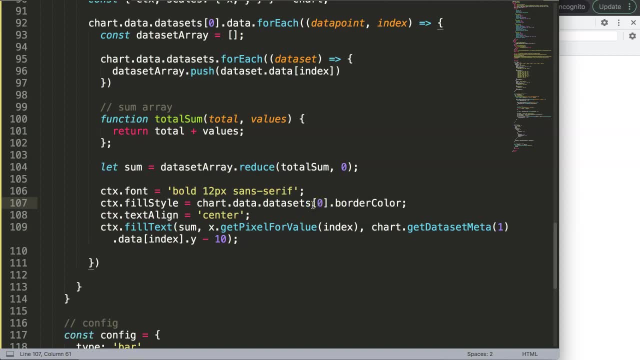 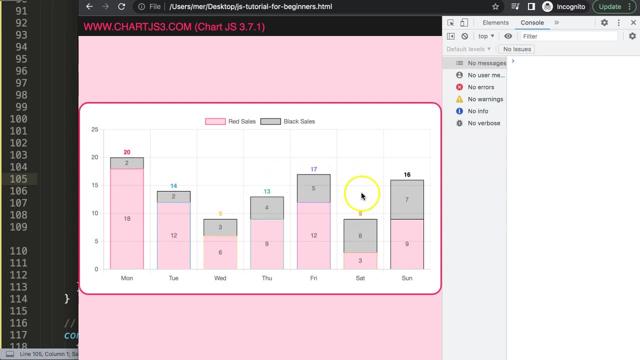 sets, then eventually say background color or border color. in our case we're going to say here: this needs to be specified as index 0, that's the one you want, border color. and then you can say your index, save that refresh, and now you can see we have all these matching colors here as well. 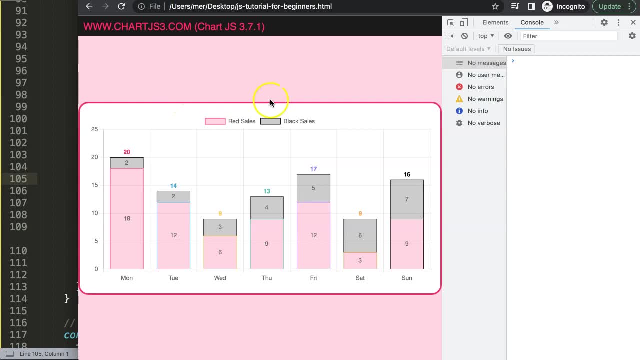 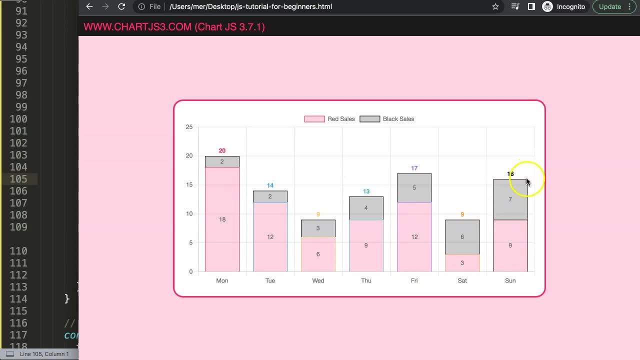 with our border and that's basically how you can play around with this. so that is completely how to do it. so maybe if you only have one item, you need to filter out an item here and i've skipped that, but because i have a whole video that explains that in here, i would highly recommend. 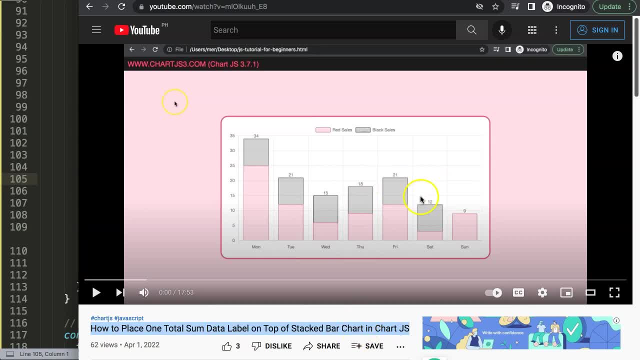 you this video here, where i use almost the same methodology, except i will use a filtering in here as well. if you understand the video, i'm going to use a filtering in here as well. if you understand on the filtering, you can apply that as well. copy that one and put it in here. if